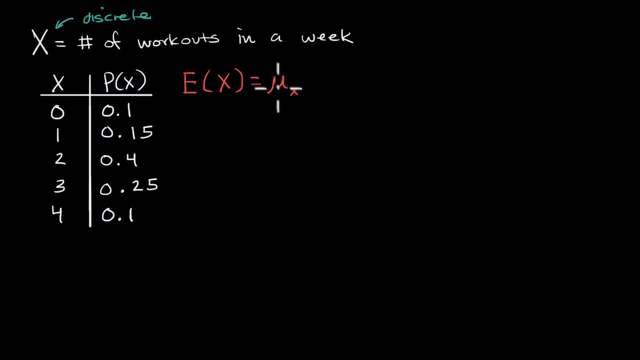 which is often used to denote the mean. So this is the mean of the random variable x. But how do we actually compute it? To compute this, we essentially just take the weighted sum of the various outcomes and we weight them by the probabilities. 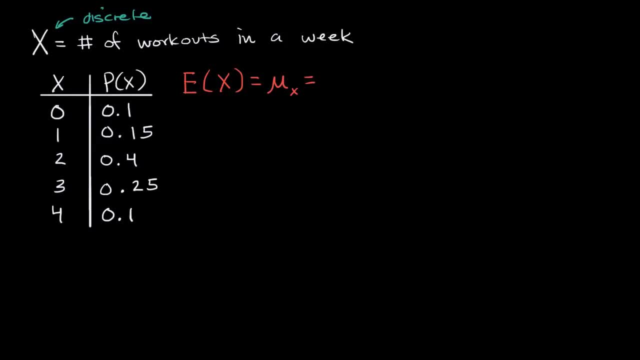 So, for example- this is going to be the first outcome here- is zero, and we'll weight it by its probability of 0.1.. So it's zero times 0.1, plus the next outcome is one, and it would be weighted by its probability of 0.15. 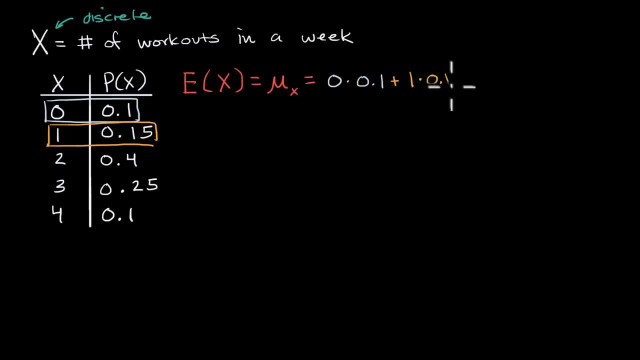 So plus one times 0.15, plus, the next outcome is two. it has a probability of 0.4, plus two times 0.4, plus the outcome three has a probability of 0.25, plus three times 0.25.. 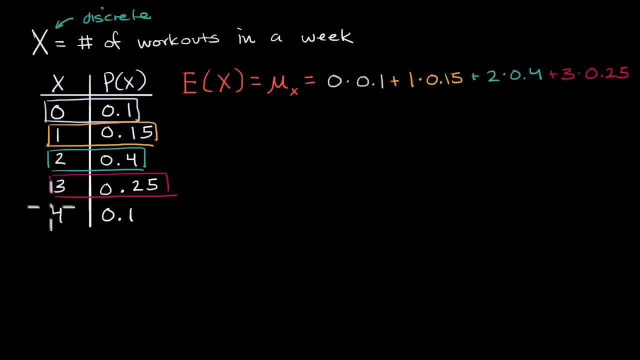 And then, last but not least, we have the outcome: four workouts in a week that has a probability of 0.1, plus four times 0.1.. Well, we can simplify this a little bit: Zero times anything is just a zero. 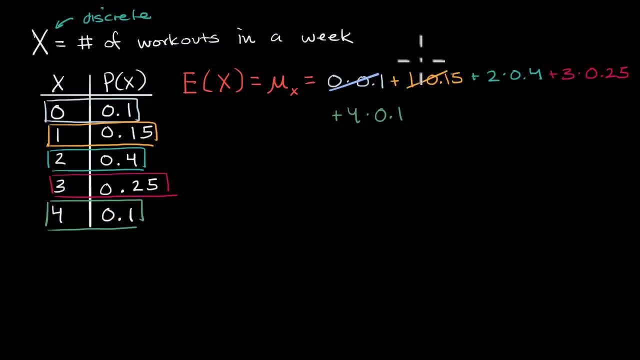 So one times 0.15 is 0.15.. Two times 0.4 is 0.8.. Three times 0.25 is 0.75.. And then four times 0.1 is 0.4.. 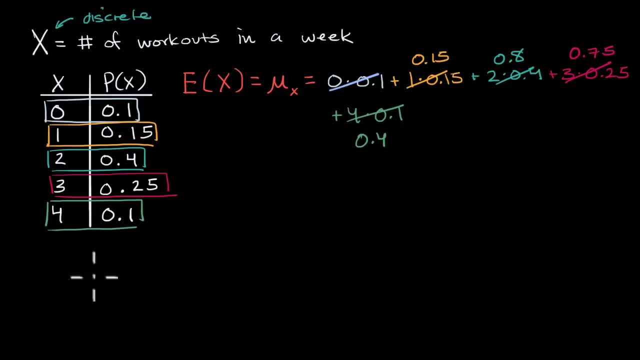 And so we just have to add up these numbers, So we get. so we get 0.15 plus 0.8 plus 0.75 plus 0.4, and let's say 0.4, 0.75,. 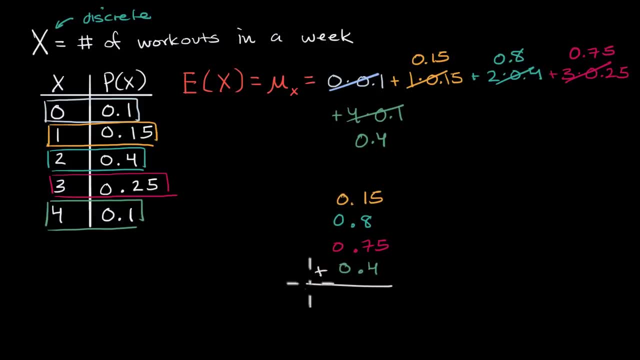 0.8.. Let's add them all together And so let's see: five plus five is 10.. And then this is two plus eight is 10,, plus seven is 17,, plus four is 21.. So we get: all of this is going to be equal to 2.1.. 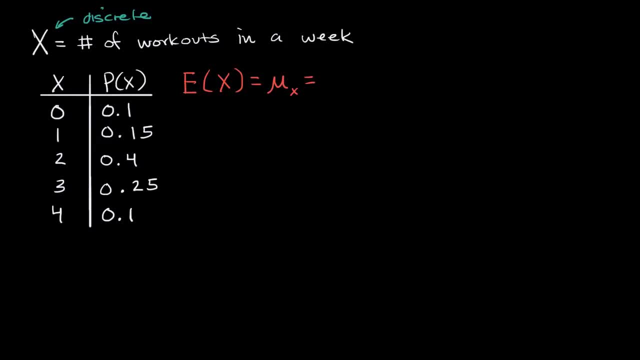 So, for example- this is going to be the first outcome here- is zero, and we'll weight it by its probability of 0.1.. So it's zero times 0.1, plus the next outcome is one, and it would be weighted by its probability of 0.15,. 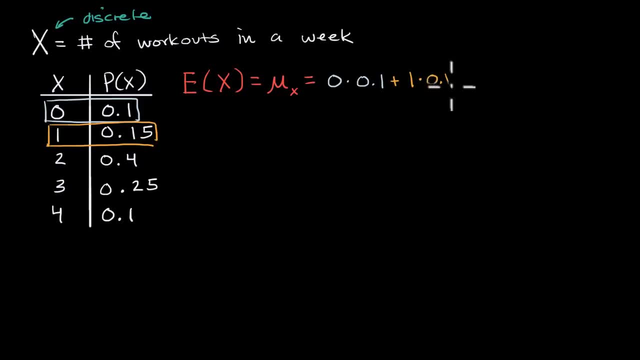 so plus one times 0.15, plus. the next outcome is two. it has a probability of 0.4, plus two times 0.4, plus. the outcome three has a probability of 0.25, plus three times 0.25,. 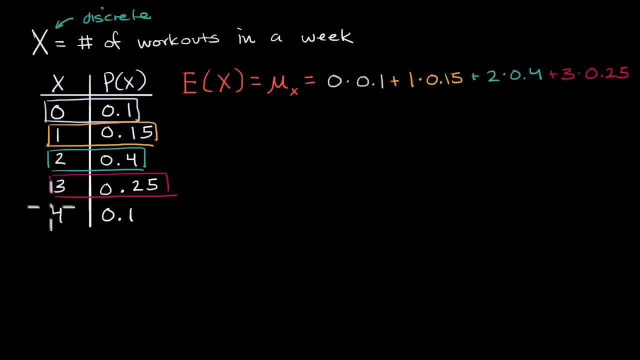 and then, last but not least, we have the outcome: four workouts in a week that has a probability of 0.1, plus four times 0.1.. Well, we can simplify this a little bit: Zero times anything is just a zero. 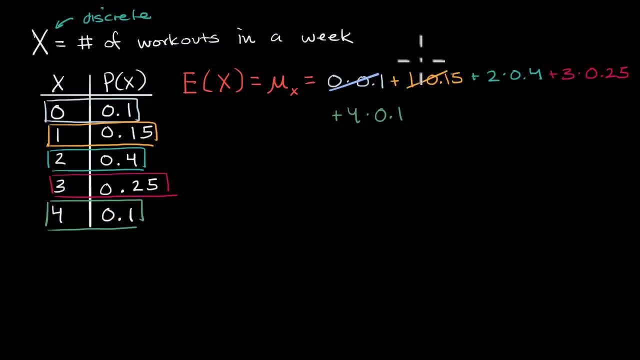 so one times 0.15 is 0.15,, two times 0.4 is 0.8,, three times 0.25 is 0.75, and then four times 0.1 is 0.4.. 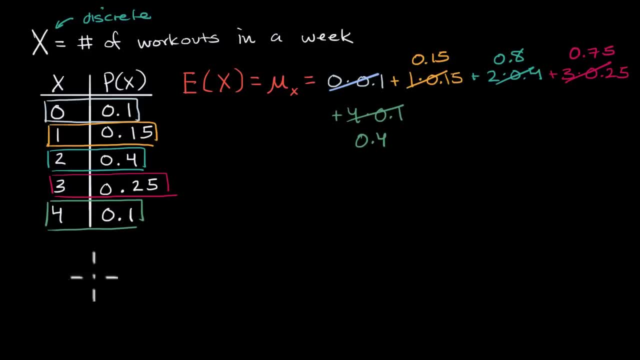 And so we just have to add up these numbers, So we get 0.15 plus 0.8 plus 0.75 plus 0.4, and let's say 0.4, 0.75, 0.8.. 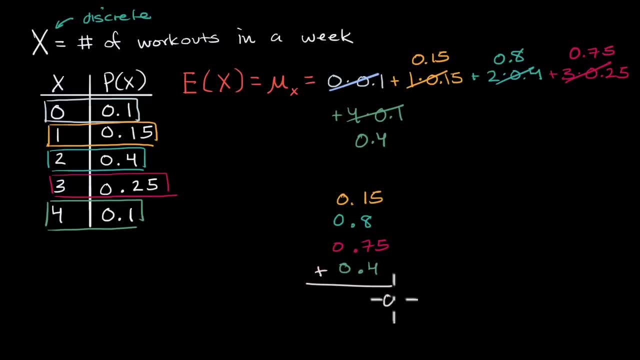 Let's add them all together And so let's see: five plus five is 10, and then this is: two plus eight is 10,, plus seven is 17,, plus four plus four is 21.. So we get: all of this is going to be equal to 2.1.. 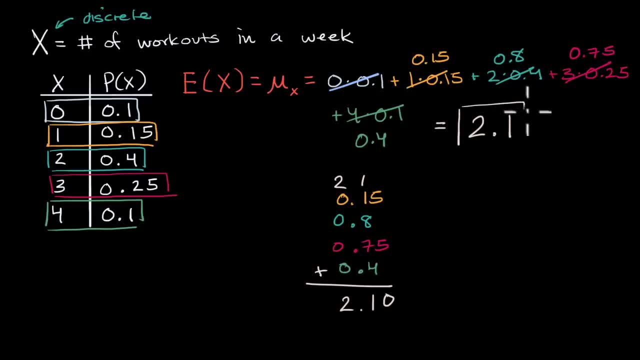 So one way to think about it is the expected value of x, the expected number of workouts for me in a week. given this, probability distribution is 2.1.. Now you might be saying wait, hold on a second. All of the outcomes here are whole numbers.